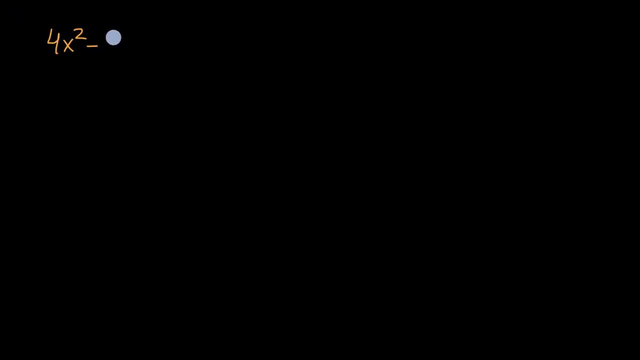 So let's see if we can try to factor the following expression completely. So factor this completely, Pause the video and have a go at that. All right, now let's work through this together. So the way that I like to think about it. 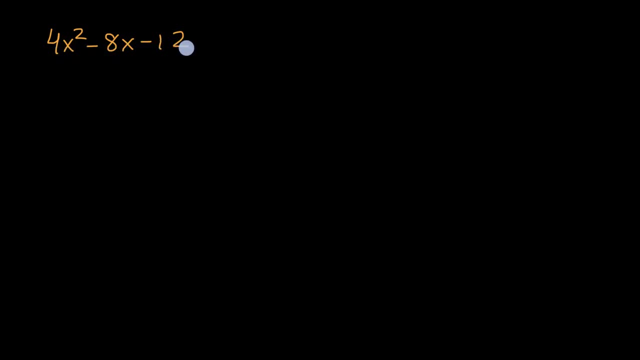 I first try to see: is there any common factor to all the terms? And I try to find the greatest of the common factor possible common factors to all of the terms. So let's see, They're all divisible by two, so two would be a common factor. 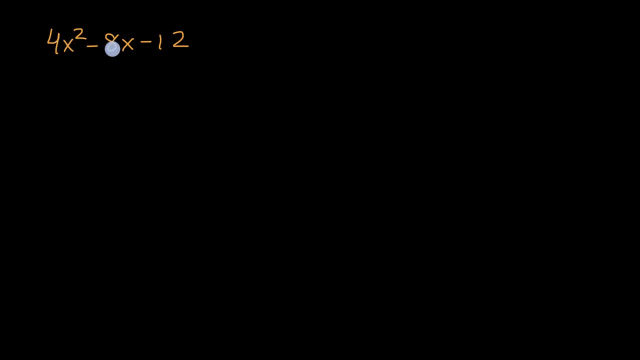 But let's see, they're also all divisible by four. Four is divisible by four, Eight is divisible by four, 12 is divisible by four, And that looks like the greatest common factor. They're not all divisible by x, so I can't throw an x in there. 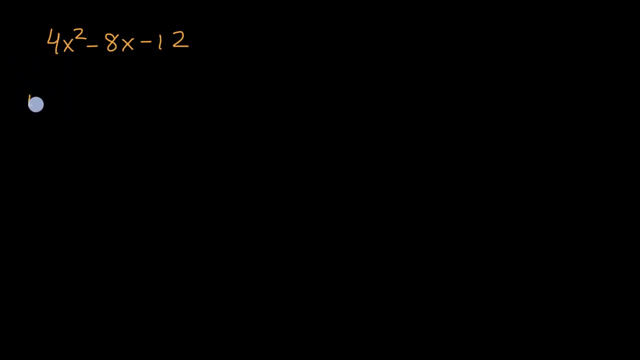 So what I wanna do is factor out a four, So I could rewrite this as four times. now what would it be? Four times what? Well, if I factor four out of four x squared, I'm just going to be left with an x squared. 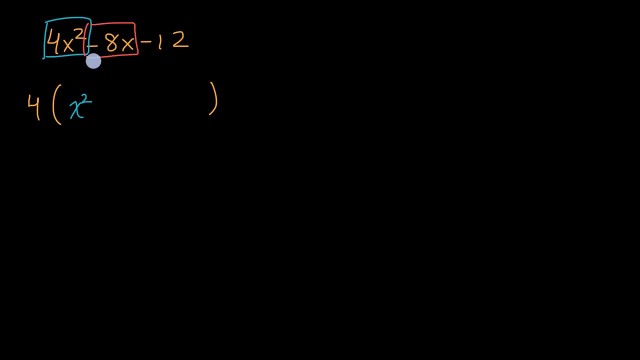 If I factor a four out of negative eight x, negative eight x divided by four is negative two. so I'm going to have negative two x. And if I factor a four out of negative 12, negative 12 divided by four is negative three. 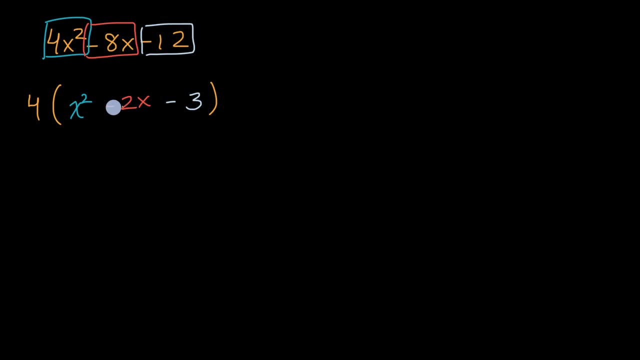 Now am I done factoring. Well, it looks like I could factor this thing a little bit more. Can I think of two numbers that add up to negative two? And when I multiply it I get negative three, And since when I multiply I get a negative value. 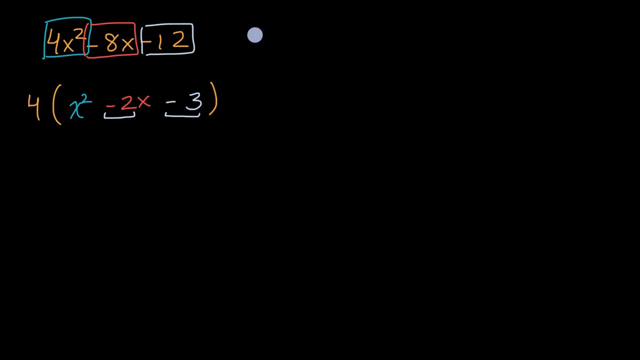 one of them's going to be positive and one of them's going to be negative. I could think about it this way: A plus b is equal to negative two. A times b needs to be equal to negative three. So let's see a could be equal to negative three. 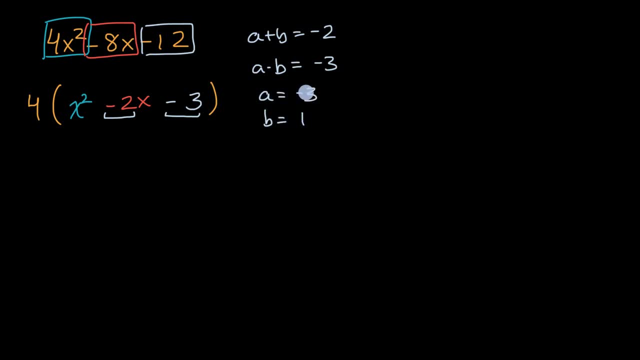 and b could be equal to one, because negative three plus one is negative two and negative three times one is negative three. So I could rewrite all of this as four times x plus negative three, or I could just write that as x minus three times x plus one. 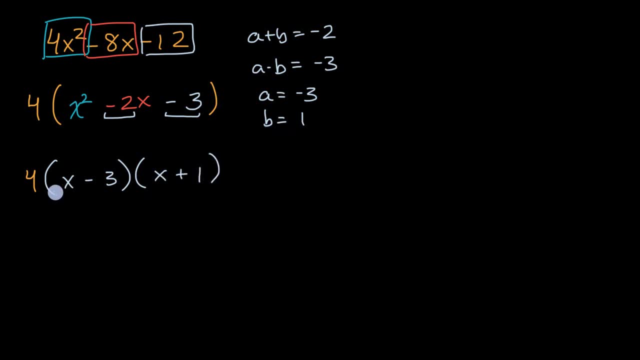 X plus one. and now I have actually factored this completely. Let's do another example. So let's say that we had the expression negative three x squared plus 21x minus 30.. Pause the video and see if you can factor this completely. 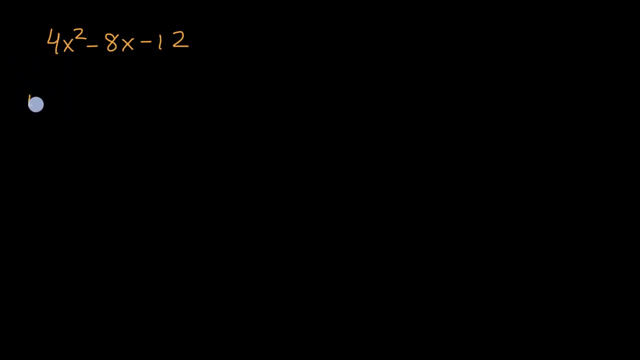 So what I wanna do is factor out a four, So I could rewrite this as four times. now what would it be? Four times what? Well, if I factor four out of four x squared, I'm just going to be left with an x squared. 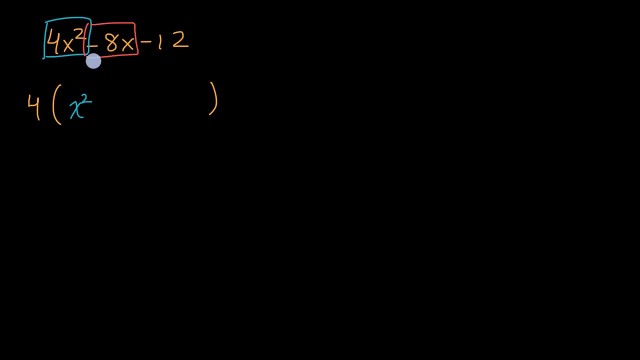 If I factor a four out of negative eight x, negative eight x divided by four is negative two. so I'm going to have negative two x. And if I factor a four out of negative 12, negative 12 divided by four is negative three. 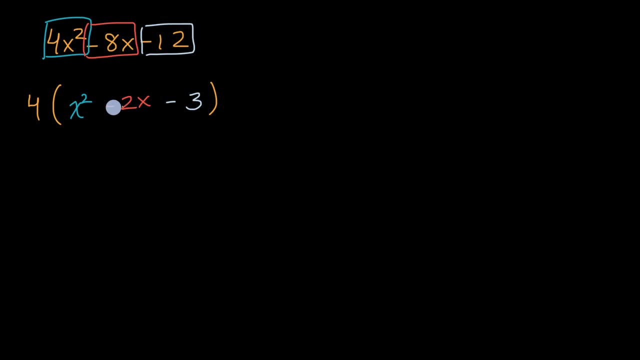 Now am I done factoring. Well, it looks like I could factor this thing a little bit more. Can I think of two numbers that add up to negative two? And when I multiply it I get negative three, And since when I multiply I get a negative value. 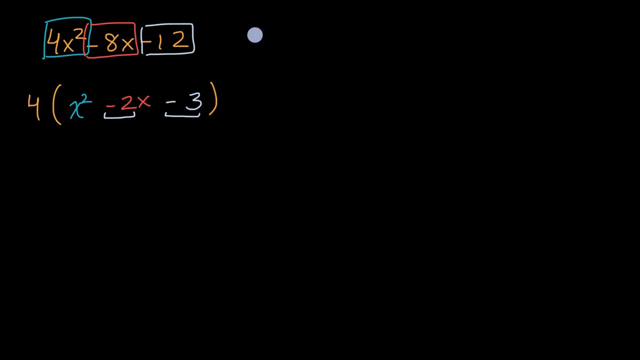 one of them's going to be positive and one of them's going to be negative. I could think about it this way: A plus b is equal to negative two. A times b needs to be equal to negative three. So let's see a could be equal to negative three. and b could be equal to one, because negative three plus one is negative two and negative three times one is negative three. So I could rewrite all of this as four times x plus negative three, or I could just write that as x minus three times x plus one. 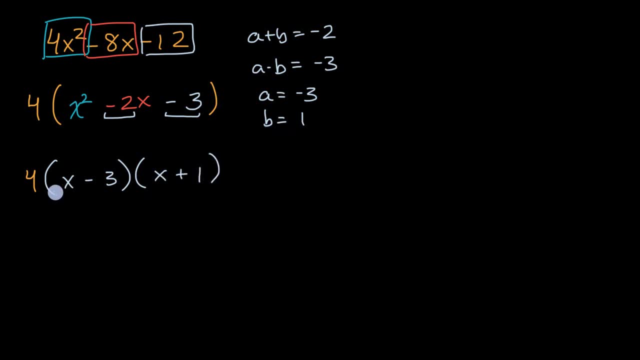 X plus one. and now I have actually factored this completely. Let's do another example. So let's say that we had the expression negative three x squared plus 21x minus 30.. Pause the video and see if you can factor this completely. 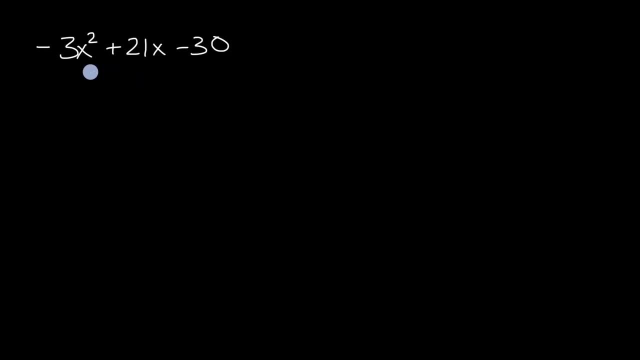 All right, now let's do this together. So what would be the greatest common factor? So let's see, they're all divisible by three. so you could factor out a three. but let's see what happens if you factor out a three. 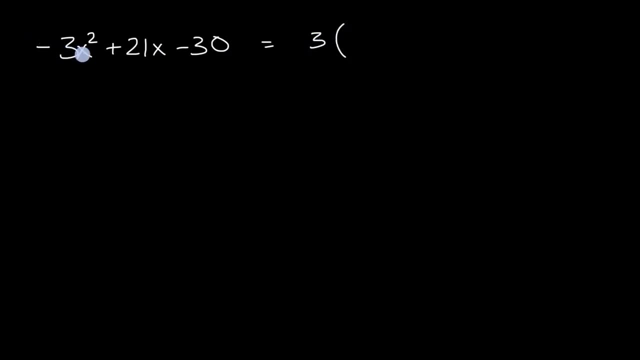 This is the same thing as three times well, negative three x squared divided by three is negative x squared 21x divided by three is seven x. so plus seven x. and then negative 30 divided by three is negative 10.. 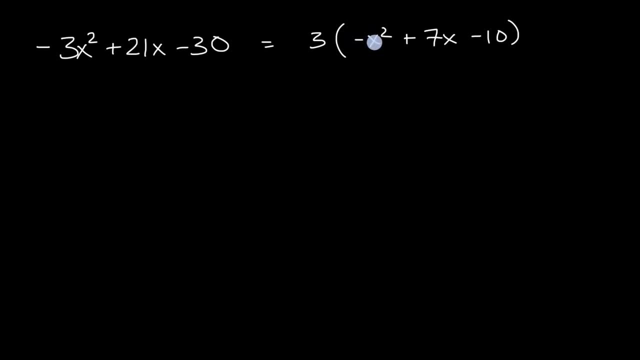 You could do it this way, but having this negative out on the x squared term still makes it a little bit confusing. on how you would factor this further, You can do it, but it still takes a little bit more of a mental load. So instead of just factoring out a three, 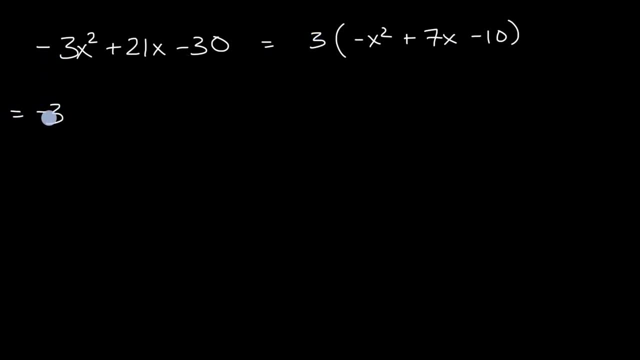 let's factor out a negative three. So we could write it this way: If we factor out a negative three, what does that become? Well then, if you factor out a negative three out of this term, you're just left with an x squared.